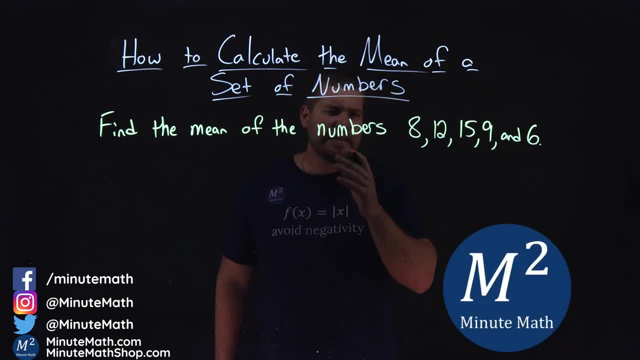 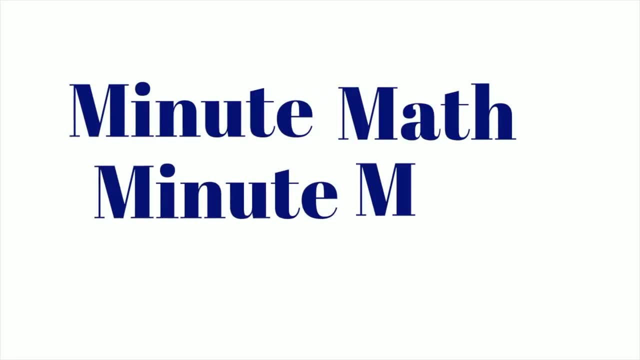 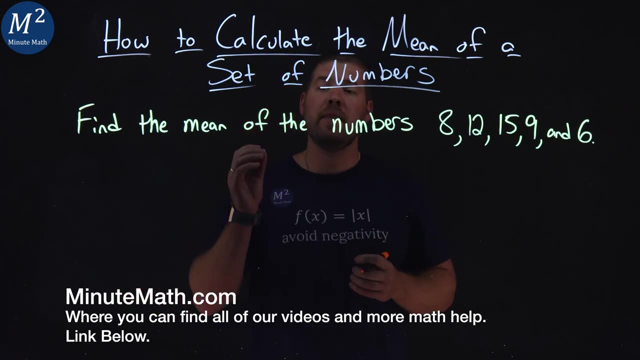 Hi, I'm Sean Gannon and this is Minute Math, and today we're learning about how to calculate the mean of a set of numbers- Minute Math, Minute Math. when you need help, you use Minute Math. We're given this problem here. We want to find the mean of the numbers 8,, 12,, 15,, 9, and 6.. 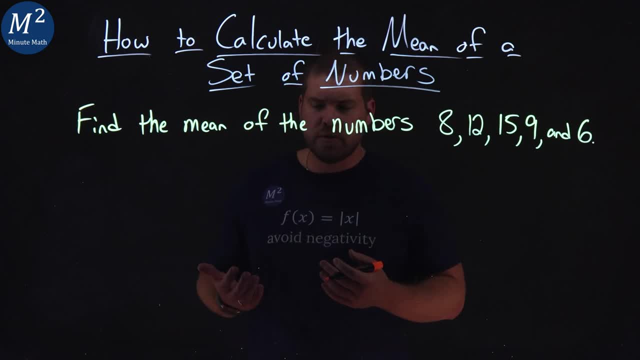 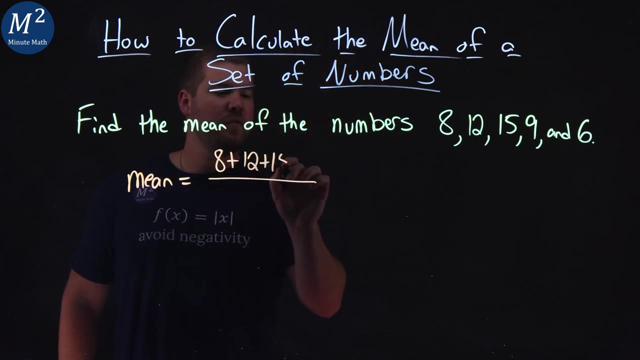 Well, the mean is also kind of known as the average. So we take our set of numbers, our mean, and we want to find that That is actually equal to the sum of all of our numbers: 8 plus a 12 plus a 15 plus a 9 plus a 6,. 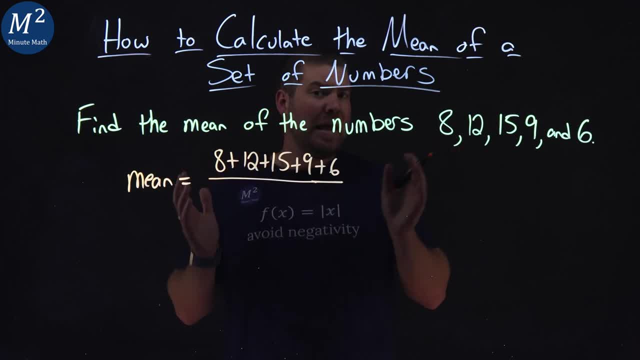 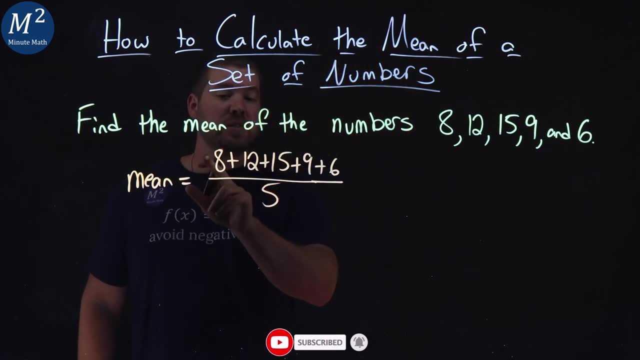 over the total numbers that we have. How many do we have? 1,, 2,, 3,, 4, and 5.. So again we have the sum Adding up all the numbers that we're trying to find, the mean of divided by how many numbers that we have. 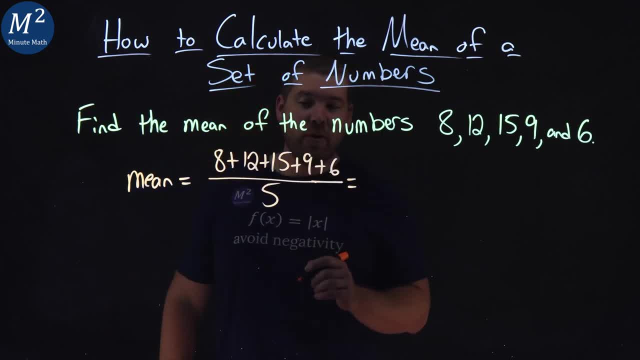 8,, 12,, 15,, 9, and 6 all added together become a 50, and we put that over 5.. Okay, Now from here. well, how did I get 50 so fast? Let's talk about that. 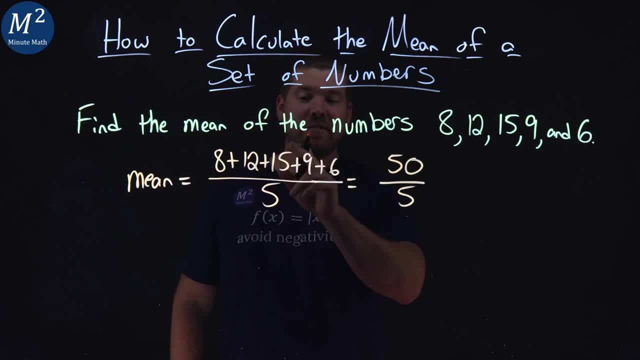 8, 12, 20.. 9 and 6 is 15.. 15, 15 is 30, plus 20 is 50. Just in case you needed to know that. But you can always take your time, I think you can add. 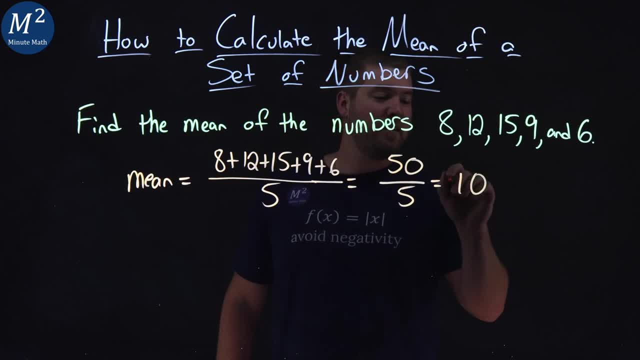 Now, 50 divided by 5, that's just a 10.. And there we have it. Our mean on the set of numbers, 8,, 12,, 15,, 9, and 6, is just a 10.. 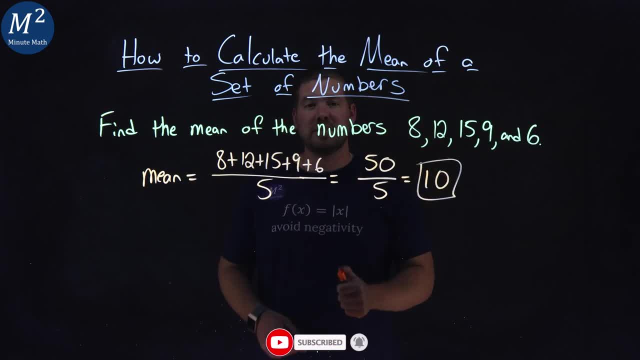 I hope you learned something here on how to calculate the mean of a set of numbers. If you did, make sure you like this video and subscribe to our YouTube channel. This helps us make more of these free math lessons for you and for everyone else. So, as always, thanks for watching.